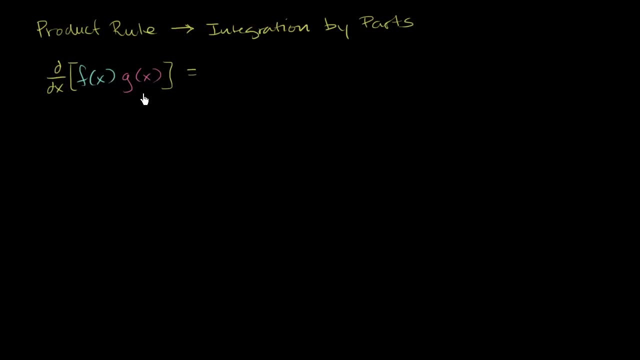 Let's apply the derivative operator right over here, And this, once again, just review of the product rule. It's going to be the derivative of the first function times the second function, So it's going to be f. No, I'm going to do that. blue color. 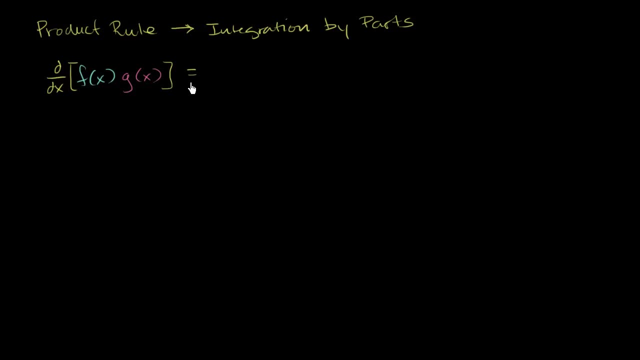 It's going to be f, That's not blue. It's going to be f, prime of x times, g of x times. that's not the same color. times g of x, g of x plus the first function times the derivative of the second. 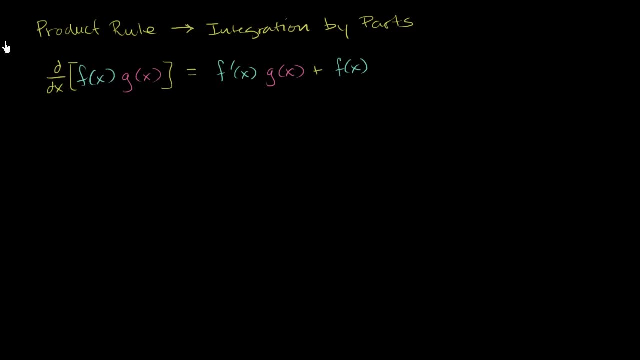 Plus the first function, f of x times the derivative of the second. Derivative of the second- This is all a review right over here- Derivative of the first times the second function plus the first function times the derivative of the second function. 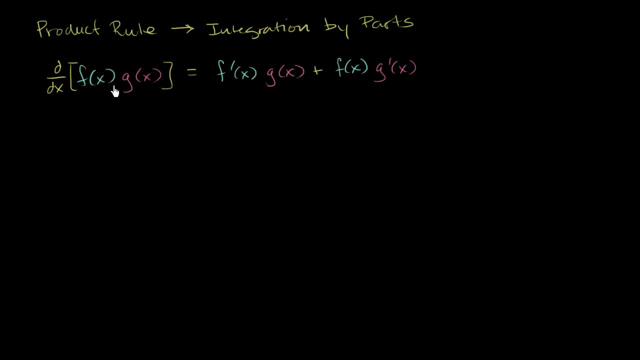 Now let's take the antiderivative of both sides of this equation. Well, if I take the antiderivative of what I have here on the left, I get f of x times g of x. We won't think about the constant for now. 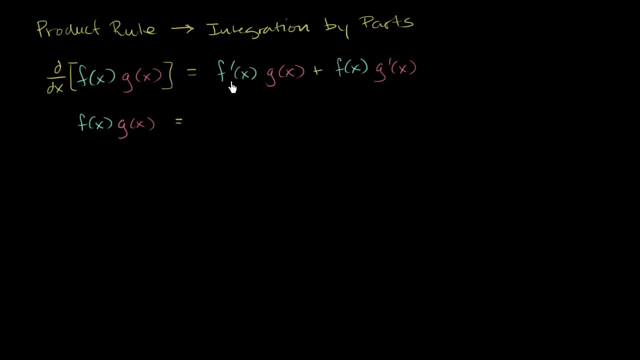 We can ignore that for now, And that's going to be equal to well. what's the antiderivative of this? This is going to be the antiderivative of f- prime of x times g of x dx, plus the antiderivative of f of x g prime of x. 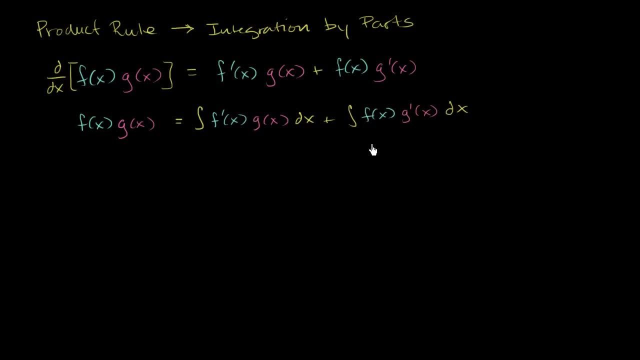 Now what I want to do is solve. I'm going to solve for this part right over here, And to solve for that I just have to subtract this business. I just have to subtract this business from both sides And then I am left with, if I subtract that from both sides. 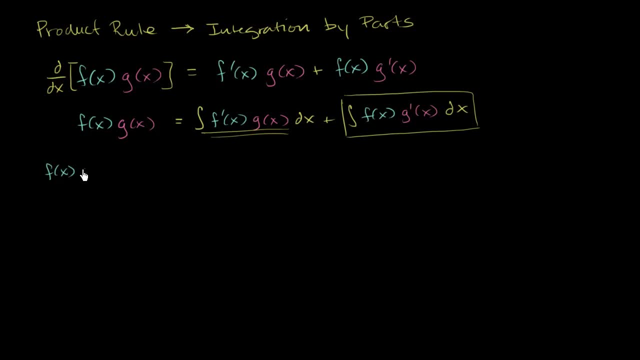 I'm left with f of x times g of x, minus this, minus the antiderivative. The antiderivative of f prime of x, g of x, g of x, g of x, dx is equal to what I wanted to solve for. 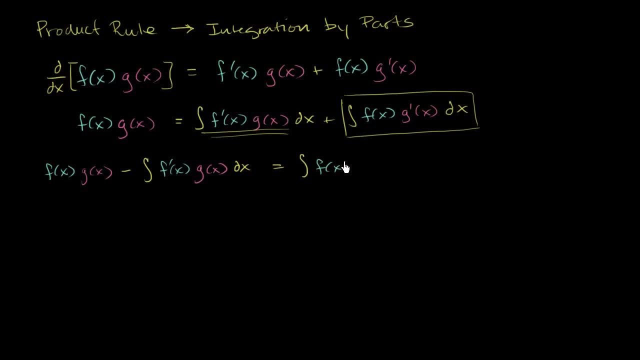 It's equal to the antiderivative of f of x g, prime of x g, prime of x dx. And to make it a little bit clearer, let me swap sides here. Let me copy and paste this. So let me copy and then paste it.